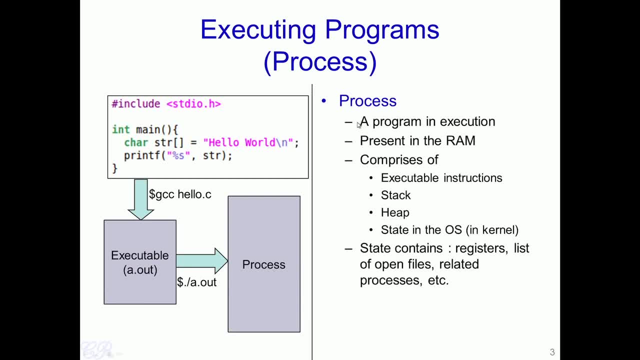 is present in the RAM. To define it formally, a process is a program under execution which is executed from RAM and essentially comprises of various sections: The executable instruction stack, heap and also a hidden section known as the state. So this state is actually maintained by the operating system and contains various things. 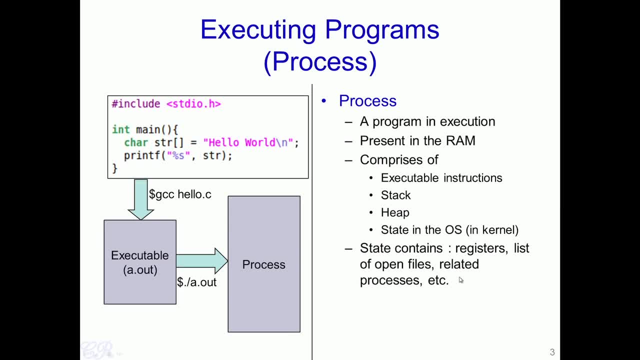 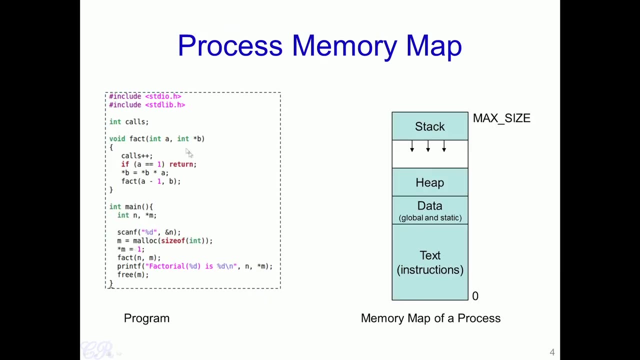 like the registers list of open files, process list of related processes, etcetera. So in today's class, we will look more into detail about what this particular process contains and how it is managed. So let us take a very simple example. So this is a. 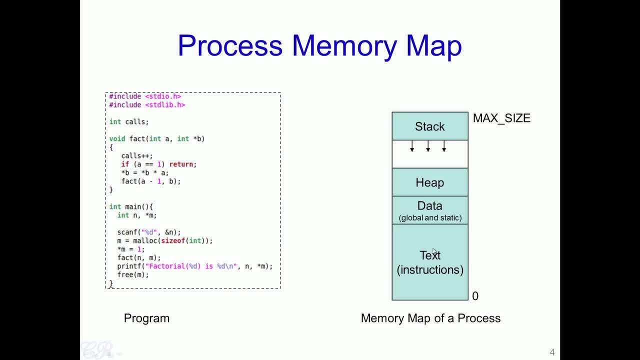 program and this is a process that is created when this program is executed. Now the process has various sections. For example, it has the text data heap and the stack. Now various parts of this program, when executed, get mapped into the various sections of the process. 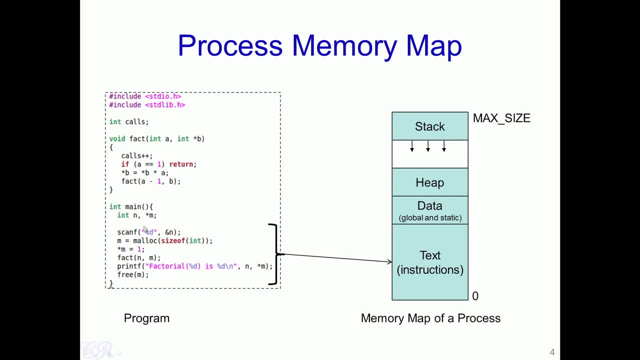 For instance, all the instructions, such as the instructions involved in the function main, will get mapped into the text section of the process. Similarly, other functions, such as the fact function over here. the instructions involved in this will also get mapped into the text section. Now the global data and also static. 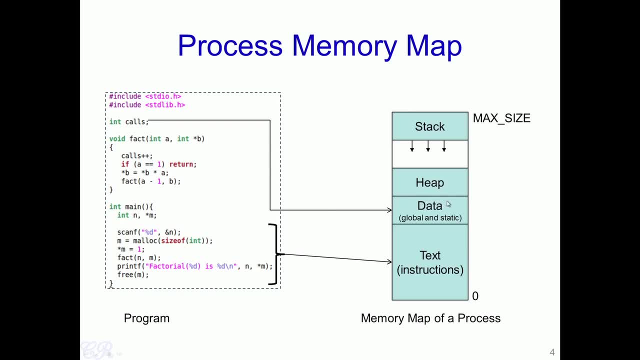 data gets mapped into the data section of the process. So this section is actually divided into two parts, called as initialized and non-initialized sections. The third section is the heap. Now any dynamically allocated memory, such as a stack, which is dynamically allocated using malloc, gets created in the heap. Now the 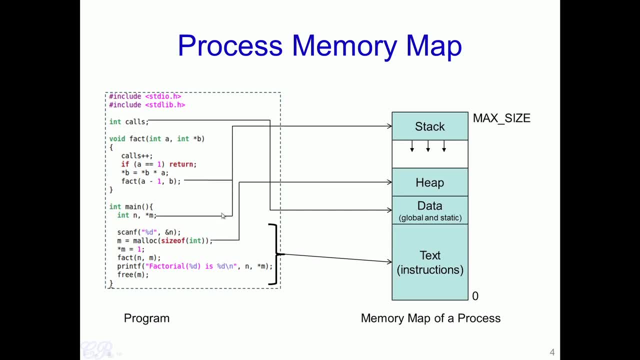 final section is called the stack, which contains all the local variables, such as n and m, and also information about function invocation, For example. in this case, we have a recursive function which is getting invoked, So all this information is present in the stack. 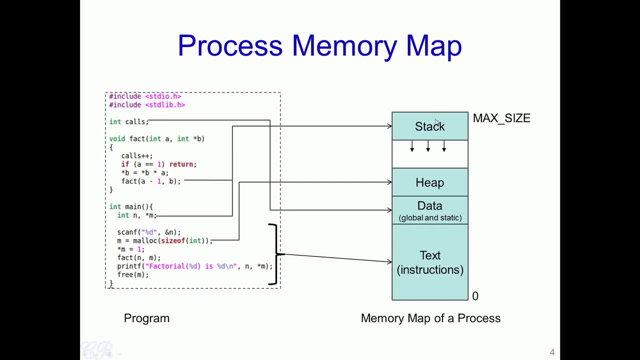 process comprising all of the sections has a maximum limit called the max size. So typically, at least in processes which are used in typical operating systems these days, this max size is going to be fixed by the OS. For instance, in a 32 bit Linux operating system, the max size for every process is: 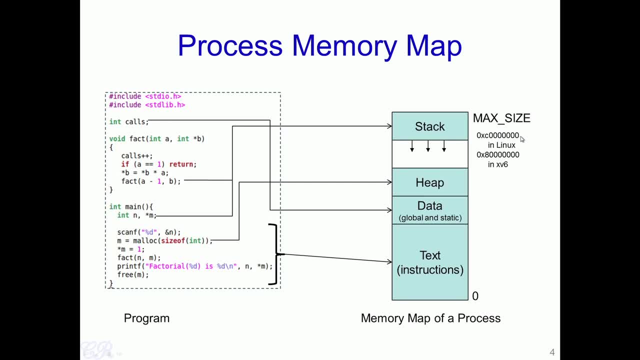 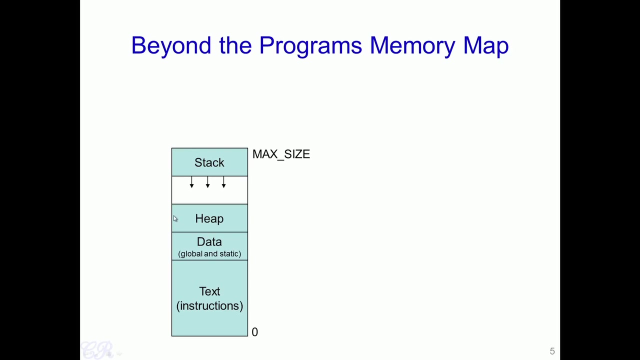 fixed at 0xc, followed by 7 zeros. In the xv6 operating system, which we are looking at for this course, the max size of a process is fixed at the address 0x8000000.. So what we had seen is that every process, a program, that is, a program under execution. 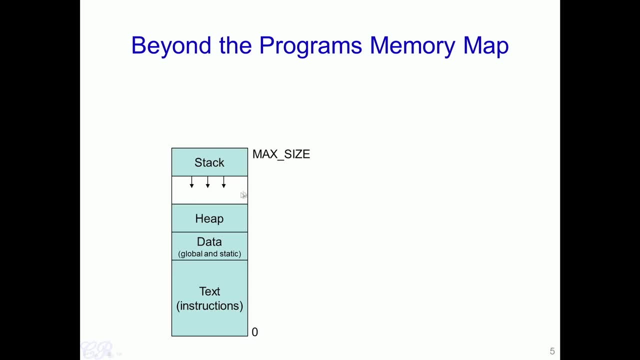 gets mapped into an area which starts at 0 and ends at max size. So what is present beyond this max size? So typically the kernel or the operating system gets mapped to the memory region from the max size to the maximum limit, The entire thing like text, that is, the instructions of the operating system. operating system. 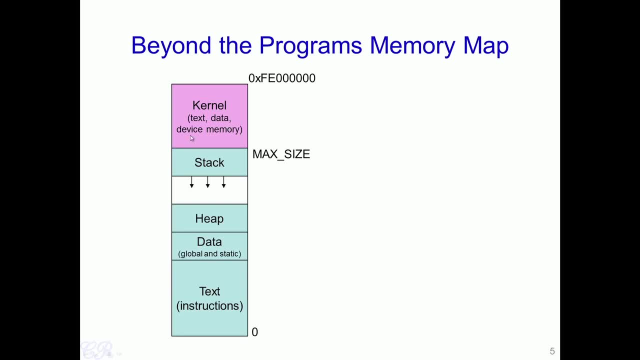 data, the OS heap and also device memory gets mapped into this upper region of the OS So typically And any user program could access any part of this lower region, that is, the green region over here. So there would not be any problem to actually read data from any of these sections, or even 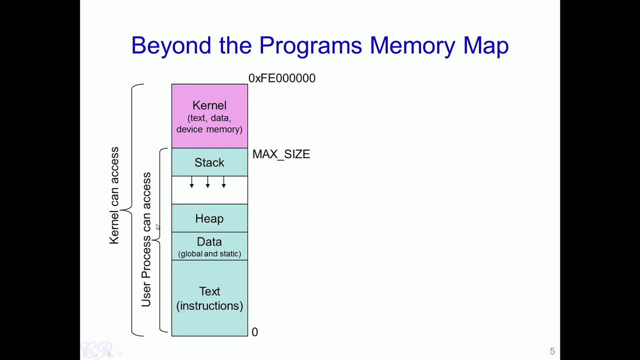 write data to parts of these sections But, however, the process cannot access any data present in the kernel memory that is beyond the max size limit. However, the kernel or the operating system which is executing from this upper region can access data from any part of the region, that is, it could execute or access data from. 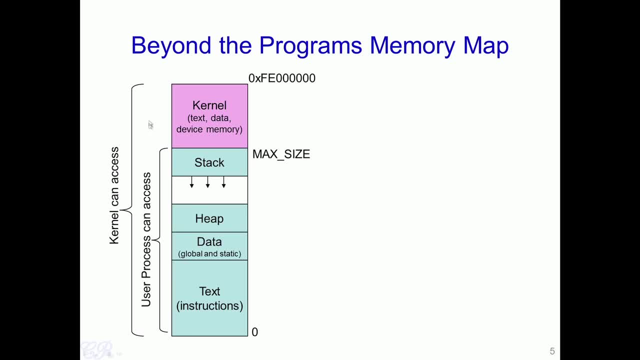 in this kernel region as well as in the user space region. Now, what happens when we actually have multiple processes running in the same system? So each process would have its own memory map, having its own instructions, data heap and stack, and also the kernel component is also present, beyond the max size. 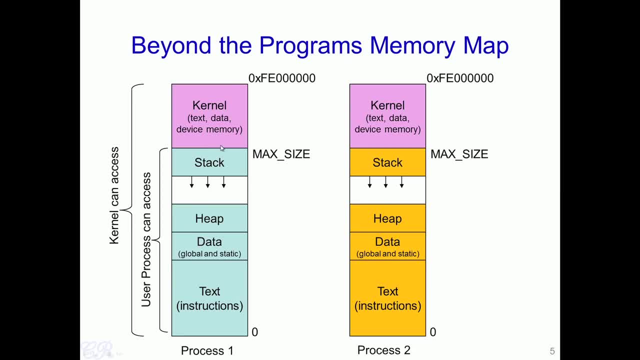 So what you see is that every process in the system would have the kernel starting at max size and extending beyond Only the lower parts, and this kernel part is going to be same for every process that is executing in the system Below this max size is going to vary from one process to another. 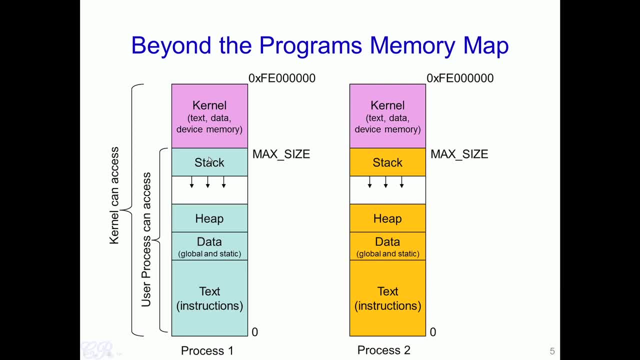 So what does this mean? So what it means is that when you execute one process and then execute another process, the regions above the max size is going to be similar, while the regions below the max size is going to change from one process to another. 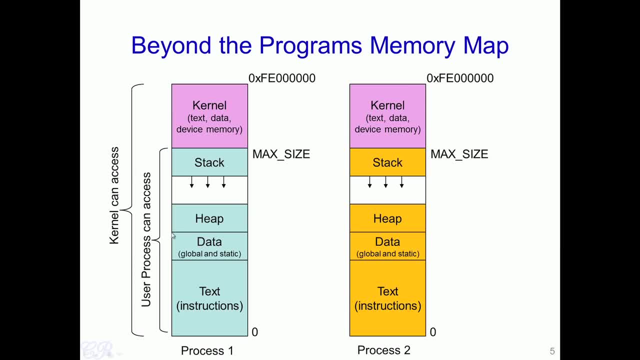 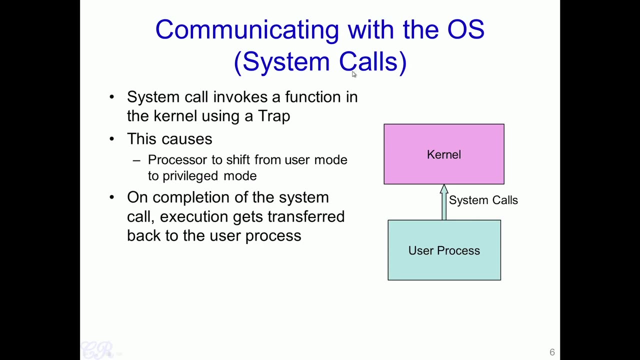 So we mentioned that user programs will not be able to access any data in the kernel space. So in that case, how does the user program actually invoke the operating system? So there are special invocation functions which the operating system support. These are known as system calls. 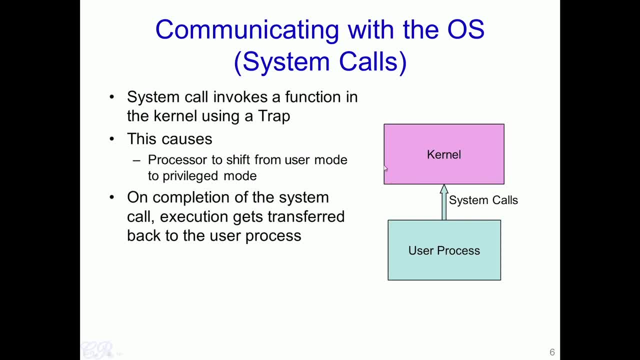 So a system calls are a set of functions Which the OS support and a user process could invoke. any of the system calls to get information or to access hardware or other resources within the kernel. So what happens when a system call is invoked? is that a process which is generally running? 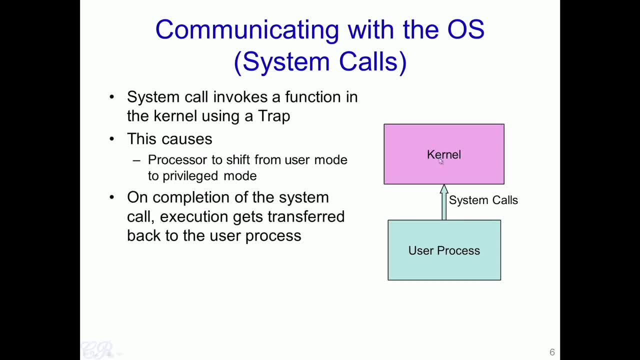 in a user mode gets shifted to something known as a kernel mode or a privilege mode, which will allow the kernel or the operating system to actually execute. When the system call completes execution, Then the user process will resume its execution from where it actually stopped. 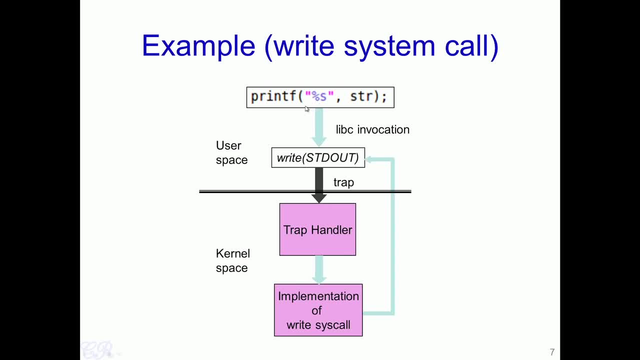 So let us take an example of the printf statement. So printf, in fact, is a library call, So it is present in this libc and it results in particular function in the user space known as write to be invoked, and this function would then invoke a system call called write, with. 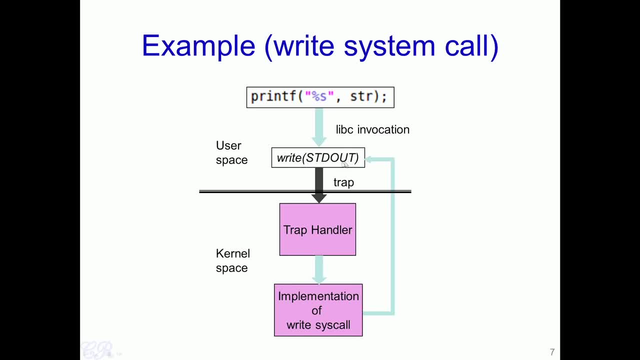 a parameter called stdout. So stdout is a special function, So it is a function which is called write. It is a parameter which essentially tells the operating system that the string provided by printf should be displayed on to the standard output, that is, the screen. 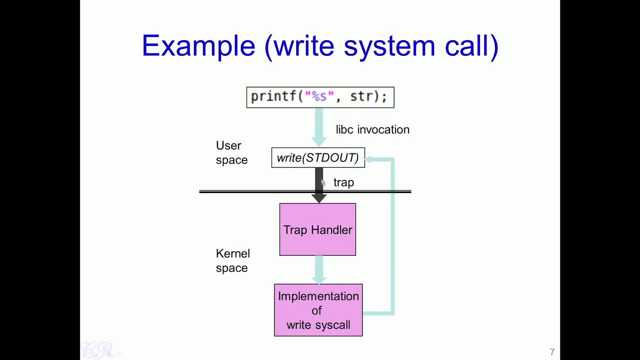 So the write is a system call which causes a trap to be triggered, and this trap will result in something known as a trap handler in the kernel space to be executed, and the trap handler would then invoke a function which will correspond to the write function. 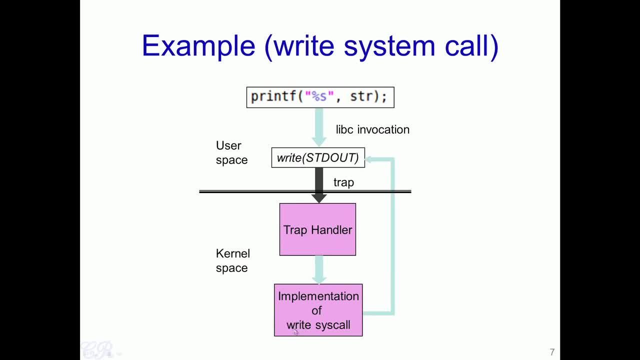 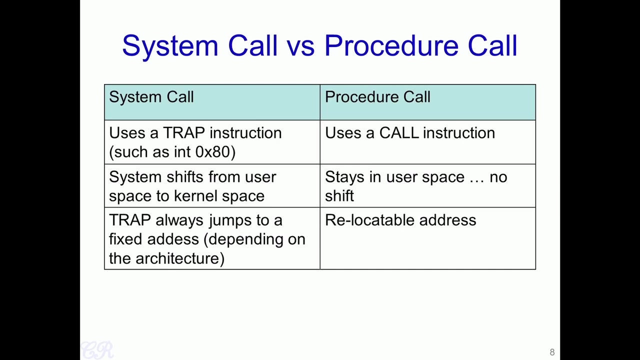 So this write system call will then be responsible for actually printing the string provided by str on to the screen. After the write system call completes, then the execution is transferred back to the user space and the process continues to execute. What is the difference between a system call versus a standard function call or procedure? 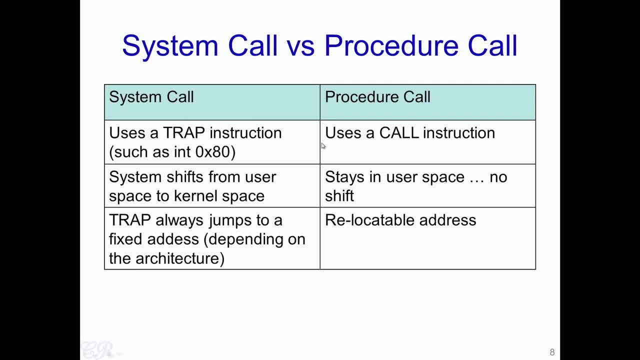 call. So? for one important difference is that when we want to invoke a function in a system call, we need to have a function called stdout. So what is the difference between a system call versus a standard function call or procedure call? So in a program or in a process we use an instruction such as a call instruction. 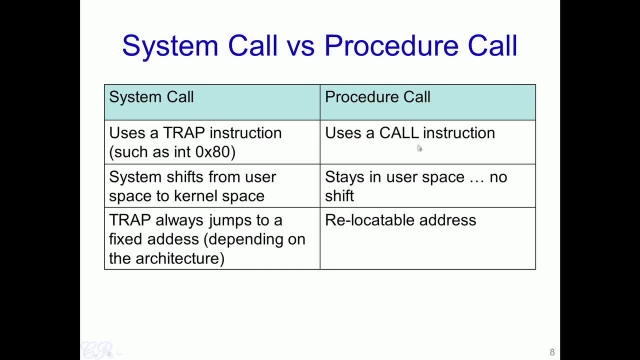 This is a standard x86 assembly instruction and this will result in the function getting called and after that function gets invoked, it returns back to the calling function. In order to invoke a system call, however, we use a trap instruction such as the int. 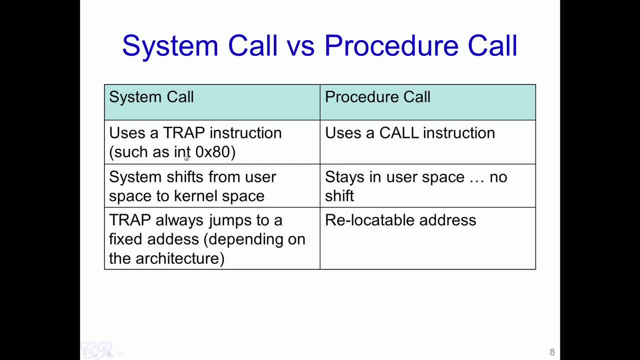 0x80.. So int here stands for interrupt or software interrupt, And it results In the system shifting from the user space or the user space mode of operation to the kernel space. So the trap instruction causes the kernel to be invoked and it causes instructions in. 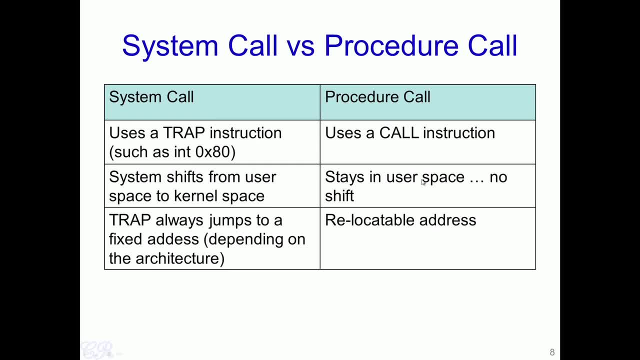 the kernel to then be executed. However, when we use the standard function call or the procedure call, using the call instruction, there is no change or shift from user space to kernel space and so on. So it the execution is done. It the execution continues to remain in the user space as it was before. 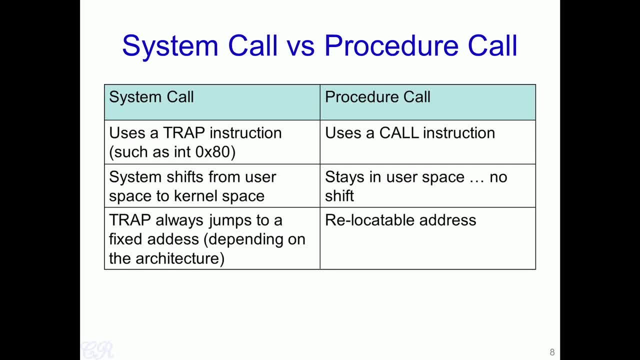 Another very subtle difference between the system call and a standard procedure call or a function call is that the destination address or the destination function which is invoked can be at a relocatable address, So it could change every time the program is compiled, and so on. 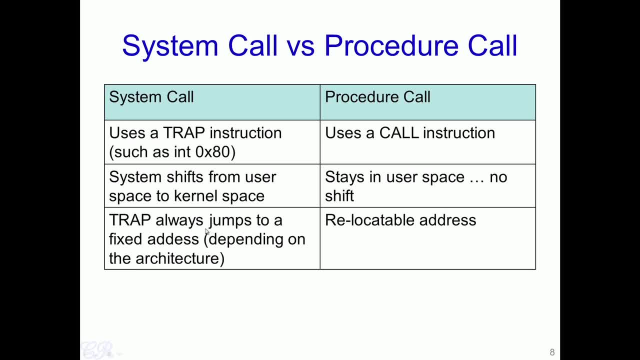 However, with the system call, when a trap instruction is used, the hardware actually or the processor, It actually decides where the next instruction in the kernel space should get invoked. So this is going to be fixed. irrespective of what program is running, what operating. 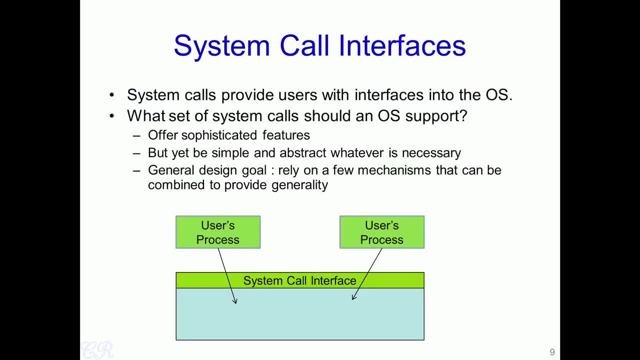 system is running, and so on. So one crucial aspect when actually designing operating systems is what system calls should the operating system supports. We had seen that the only way a user process could invoke a particular functionality in the operating system is through the system call interface. 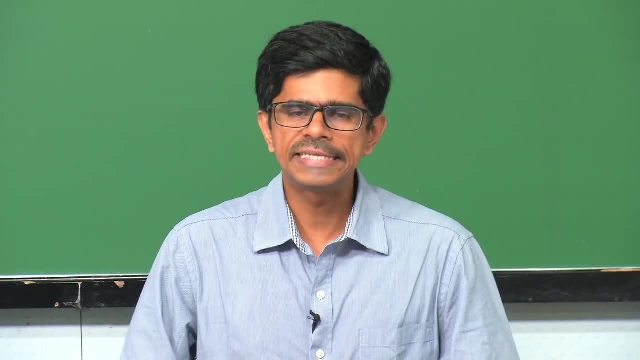 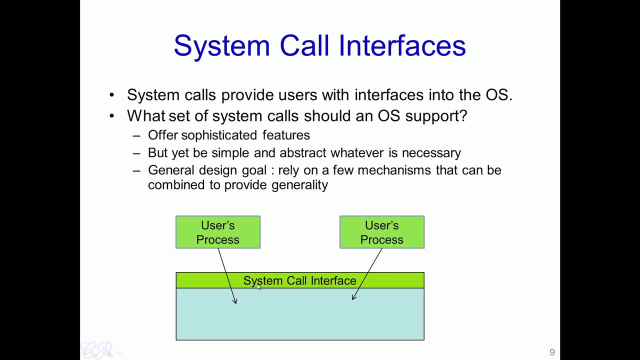 So the question now comes that if a person is actually designing an operating system, so what are the interface that the system call should support? So one obvious requirement is that the system call interface should have several sophisticated features so that a user process could actually very easily be able to interface or invoke. 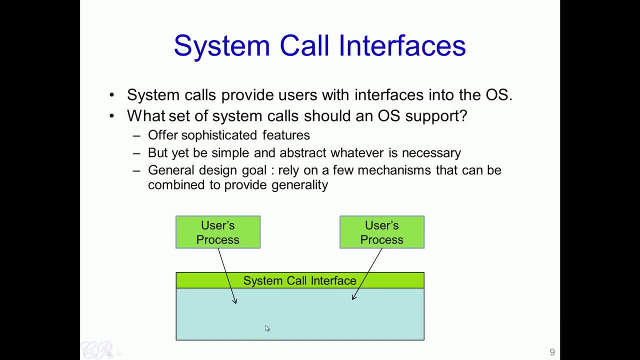 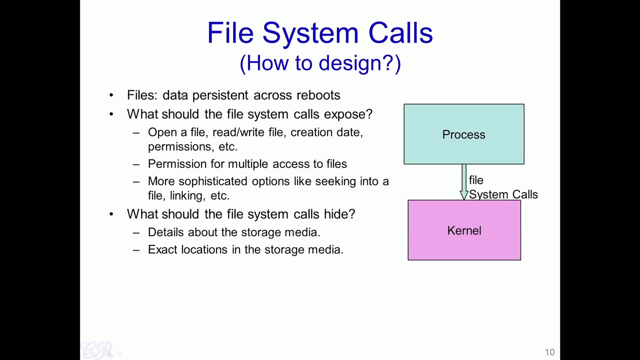 several important functionality in the operating system. However, a different approach is to have a very simple system call interface and abstract whatever is necessary from the operating system. So we will see in the next slide a particular example in this. Let us take an example of system calls that an OS supports for accessing files. 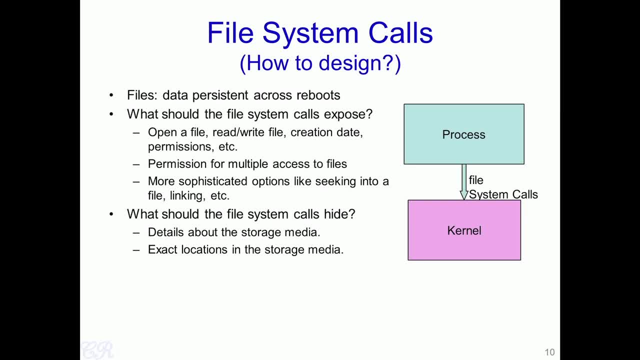 So, as we know, files are data which is persistent across reboots. So these are data which is stored in the hard disk. It could be read, written or accessed using functions such as fopen, close, read, write, and so on. 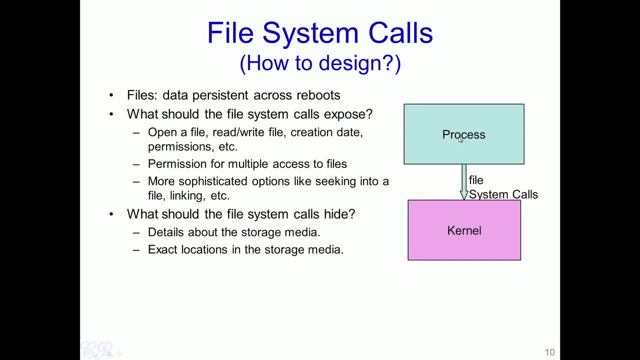 Every time we do an file open, it would require that the hard disk be accessed, So a process would need to invoke a system call into the kernel, and the kernel should actually take care of accessing the hard disk or hard disk buffers or any other storage. 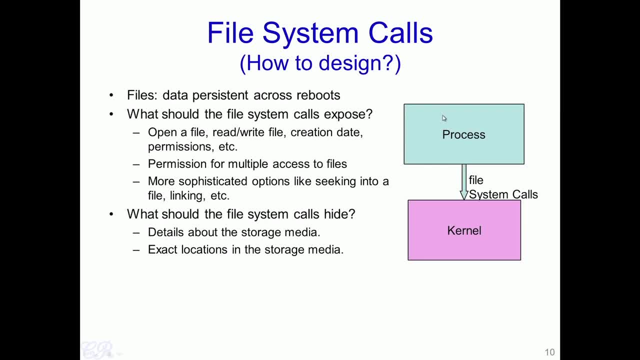 medium to open the file and return back a pointer to the process. Now the question. Now the question comes is: how does a operating system designer decide what system calls should be provided or supported in order to access files? So some of the obvious things are like there should be system calls to open a file. read 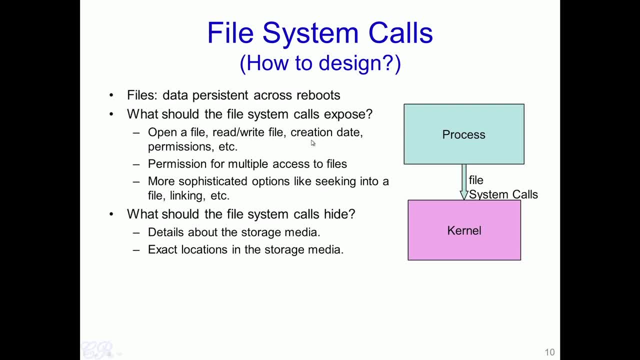 or write to a file. there should be system calls to actually modify the creation date, set permissions and so on. The operating system could also support more complicated or more sophisticated operations, such as being able to seek into a particular offset within a file, be able to link between files. 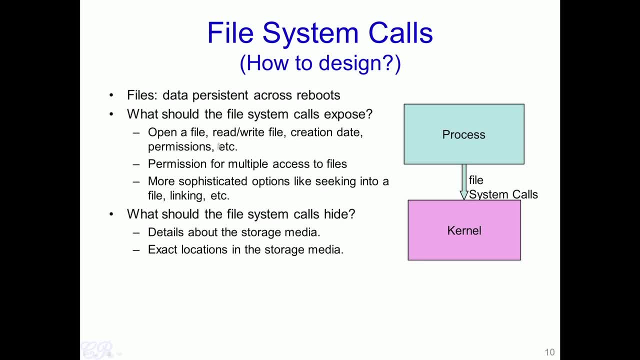 and so on. So these are the essential requirements that a system call for handling files should support. On the other hand, operating system should be able to hide some details about the file, For instance, details which should not be supported by system calls. is like things such 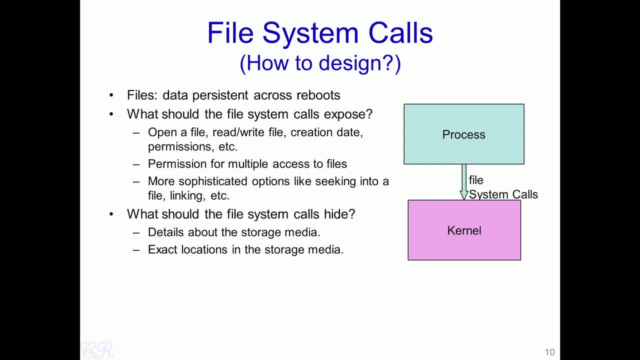 as like details about the storage media where the file is stored, For instance, whether the file is stored on a USB drive or a hard disk or a CD-ROM. This is actually abstracted out by the operating system and the user process would not be easily. 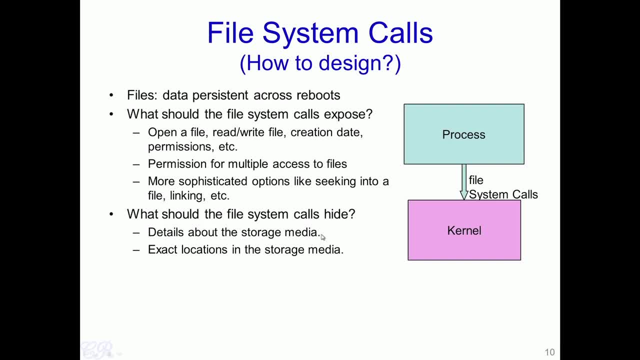 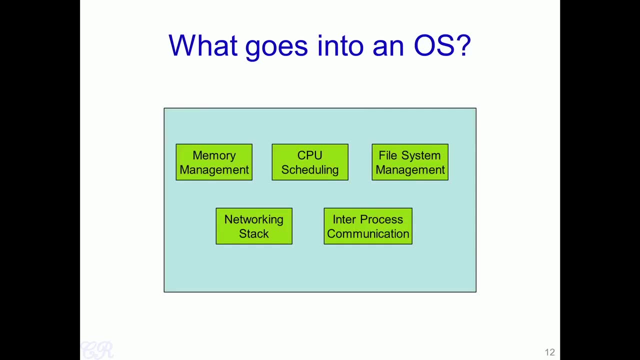 able to know where the file is stored. Another aspect which is abstracted out by the operating system is the exact locations in the storage media. We will now look at how a typical operating system works. What does the operating system structure looks like? So the operating system? suppose we consider this as this big green block- have several 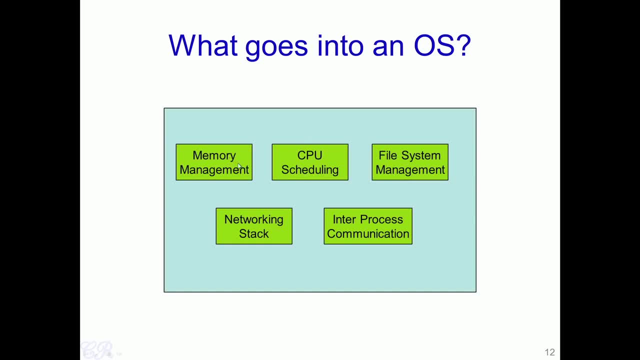 modules built internally. For example, it would have a memory management module which manages all the memory in the system. It would have a CPU scheduling block. There is also the file system management module, which will control how the file systems, such as those present in hard disk or CD-ROMs, are managed. 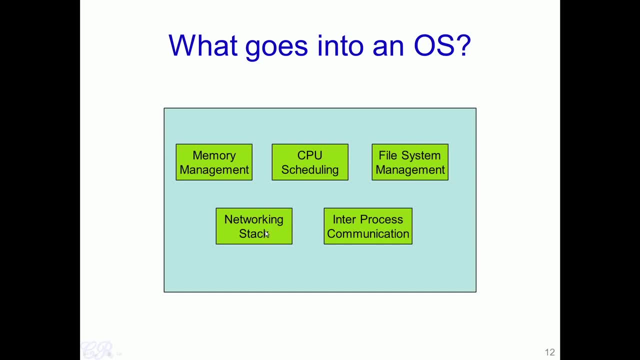 So you have a networking stack which manages the TCP IP network and you have something known as the inter-process communication module, which would take care of processes communicating with each other. So two important things which have not been mentioned as yet is the system call interface. 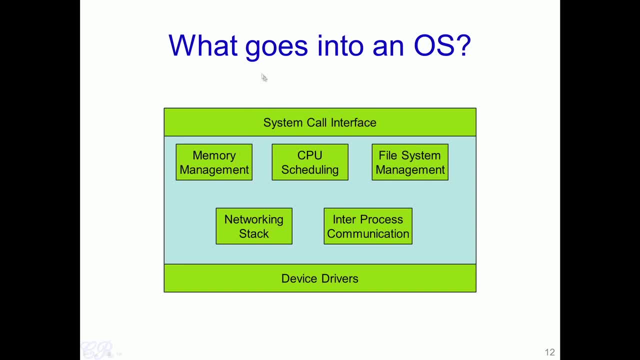 which allows user processes to actually access features or functionalities within each of these modules. Another aspect is the device drivers, which would take care of communicating with the hardware devices and other hardware resources within the system. So this, essentially, is all the different modules that an operating system supports. 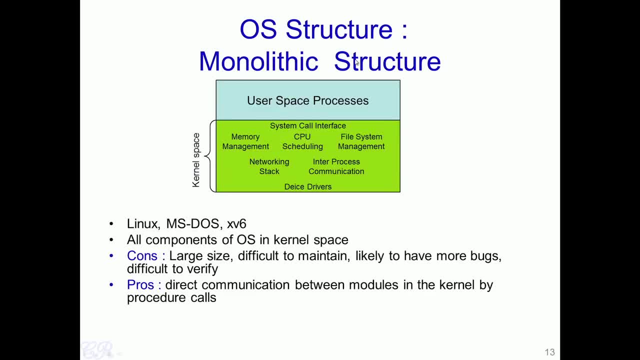 So in a monolithic structure of an operating system, all these various modules in the OS are present in a single addressable kernel space. So what this means is that this is just one large chunk of code. 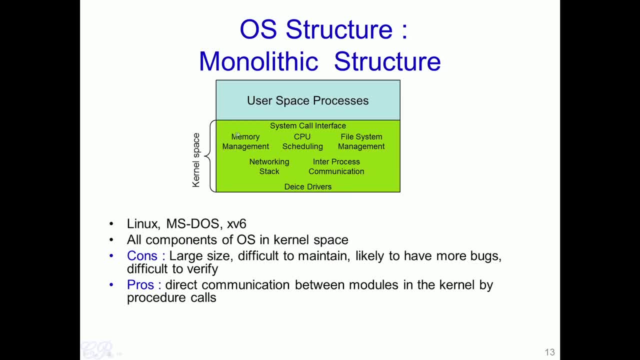 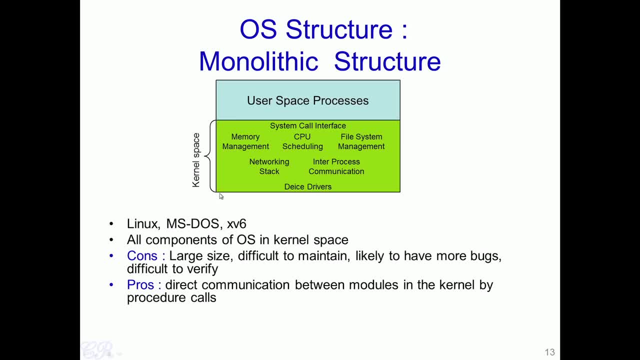 other hand, the kernel space becomes very large So and therefore difficult to maintain and is likely to have more bugs. So a typical operating system such as Linux and xv6 and MS-DOS, uses a monolithic structure. So, to take an example, the Linux operating system. 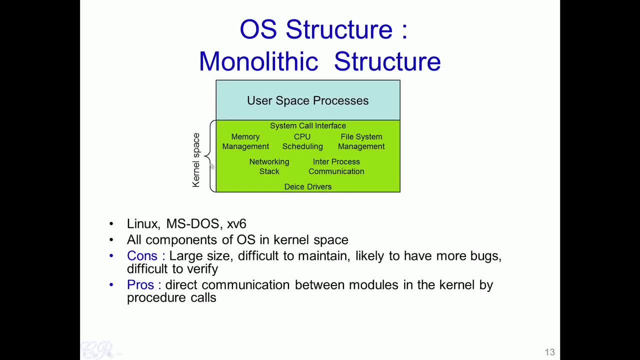 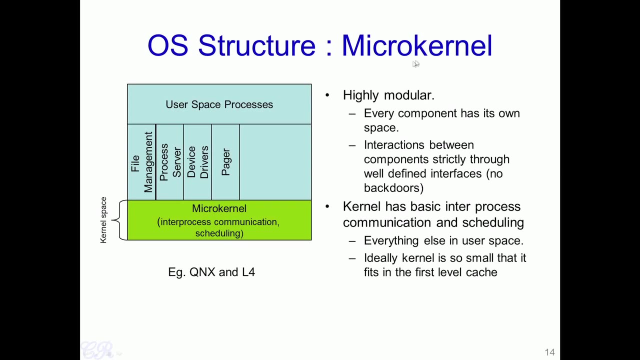 or the Linux kernel, has around 10 million lines of code. So all these 10 million lines of code comprises of the entire kernel, Linux kernel, which is actually present in this area. Another common structure of the operating system is known as the microkernel structure. 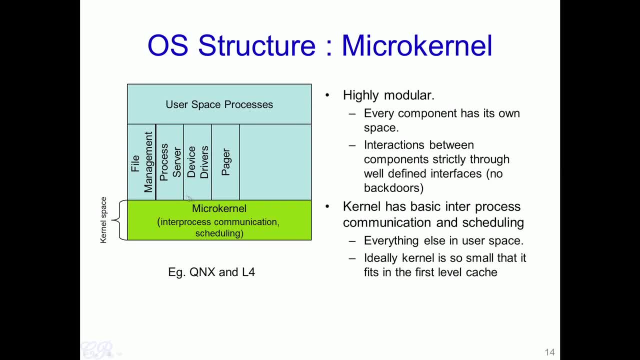 where the kernel is actually highly modular and every component in the kernel has its own addressable space. So it is like having each of these as independent processes and you have a very small microkernel which actually runs in the kernel. So, yes, the kernel space which is in charge of managing communication between each of 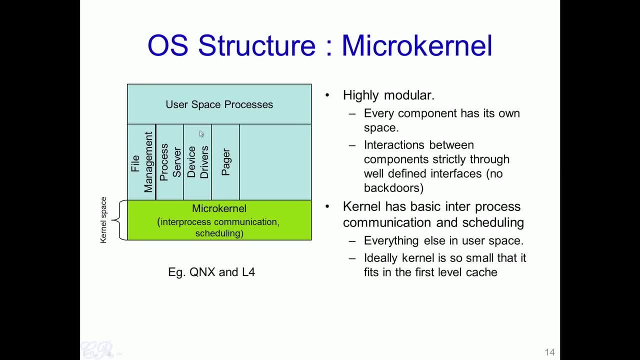 these processes and also communications between the user process and the operating system processes. So the advantage here is that this microkernel is extremely small, So ideally it is small enough to actually fit into the L1 cache of the system itself. So typically, 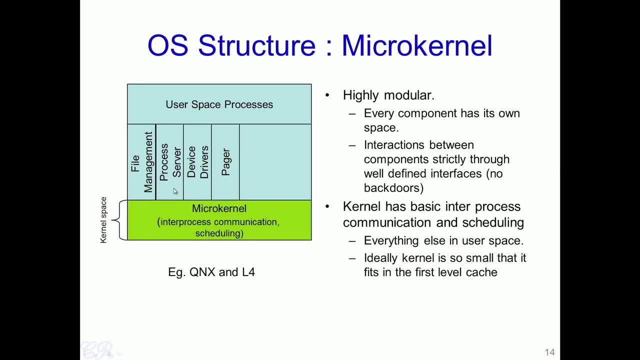 it would be quite fast. However, the drawback is that it has a little bit more space in. You now cannot have direct calls from, say, the file management to a device driver, or rather like unlike the monolithic kernel where you could make direct function invocation from a file management module to a device driver function.